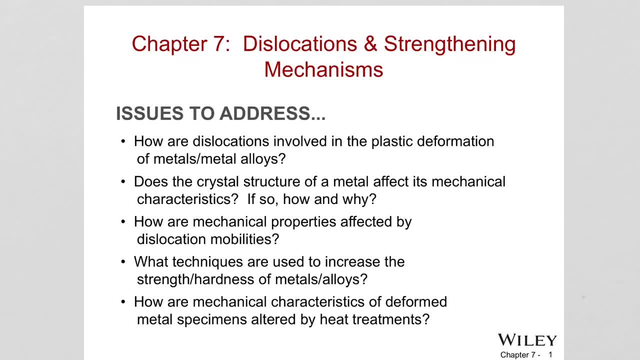 all right, guys. so in chapter seven we're gonna learn about more about the dislocations and strengthening mechanisms. so I told you before how important the dislocations are when we were looking at the defects in metallic structures, and I told you also the reason the materials can. 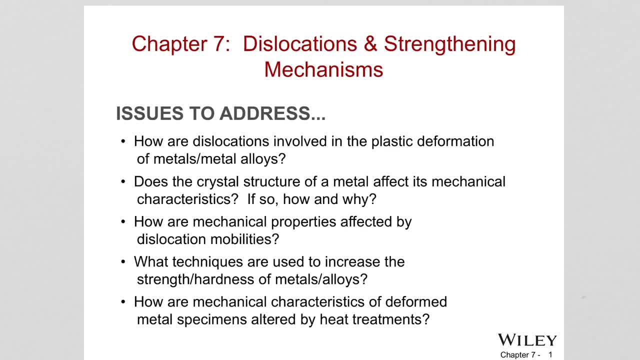 deform plastically, meaning permanently, is because of the existence of dislocations. so we're gonna learn how. what is the relationship between dislocation and the deformation? and also we're gonna learn, learn how the crystal structure of a metal affects the mechanical properties, like if it's BCC, FCC, HCP. is there a difference depending on the crystal structure? 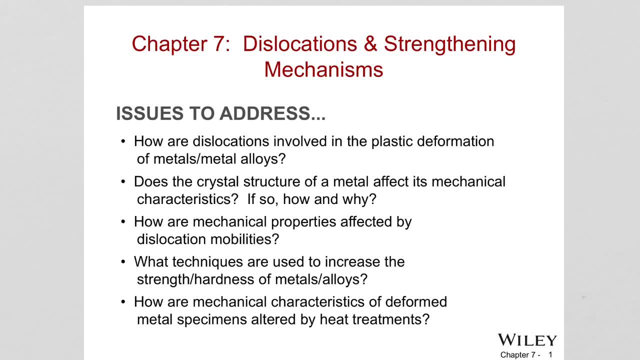 and the behavior? and if there is, then why. And then dislocation motion affects all kinds of mechanical properties, just not only strength. Okay, so we're going to learn this relationship between the dislocation motion and mechanical properties. So, with that knowledge in mind, then, how can we increase the strength and hardness of metals or their alloys? because at the 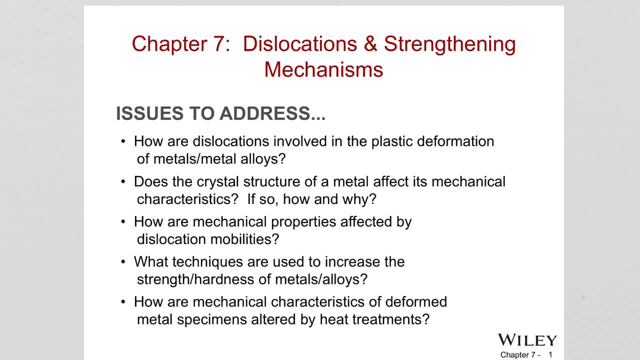 end. I know dislocations are responsible for plasticity. If I don't want plastic deformation, permanent change shape, and if I don't want my material to change shape permanently or wanted to require more strength, then how should I do? basically, how can I increase the strength and hardness And after that we're 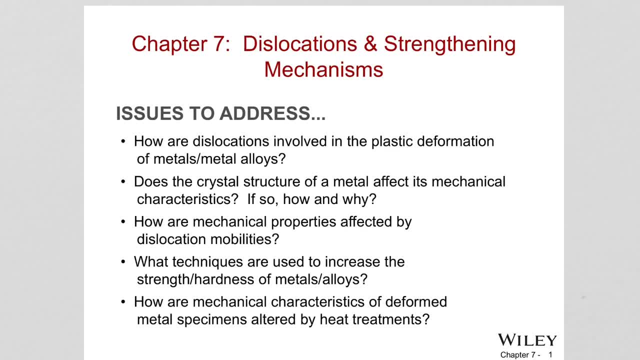 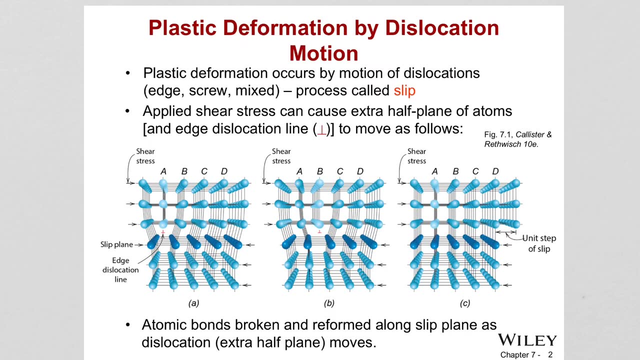 gonna see. we can also change mechanical properties by heat treatments and we're going to see how heat treatments work and how to change them affect the properties. so I guess I told you this before. but for plastic or permanent deformation to happen, because we know there is elastic deformation by stretching the bones between, and it is.